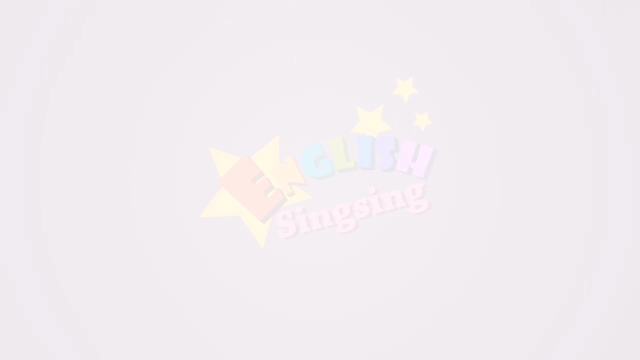 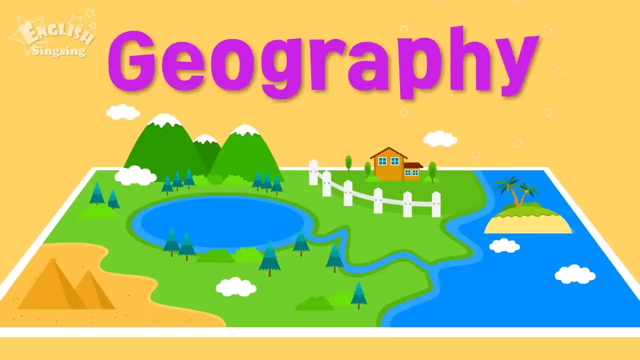 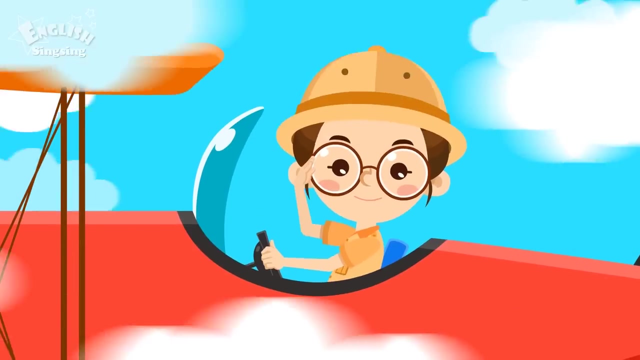 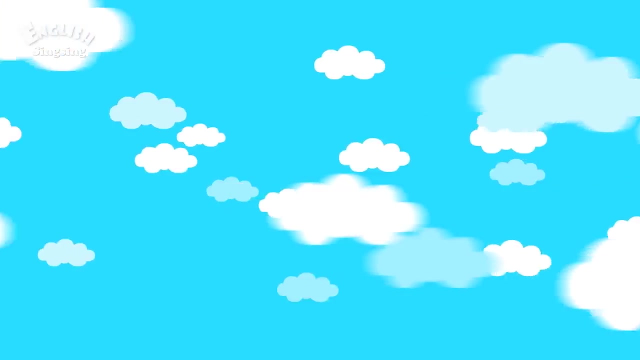 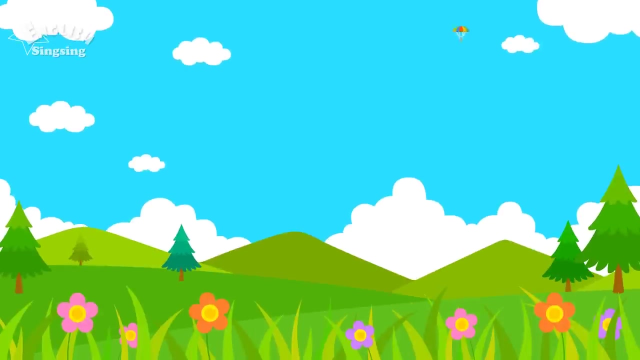 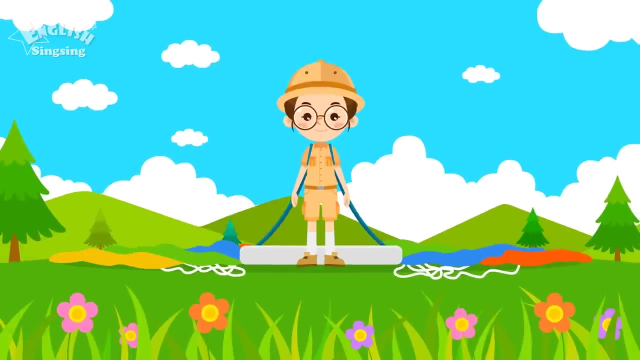 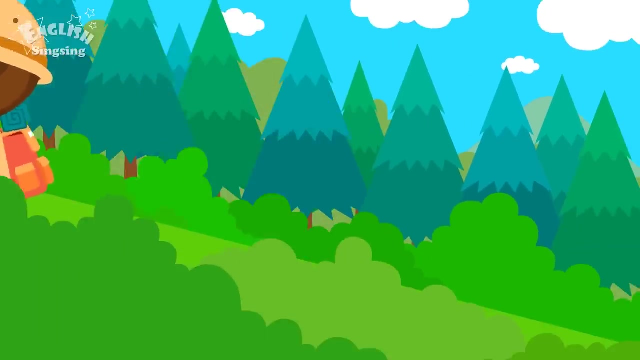 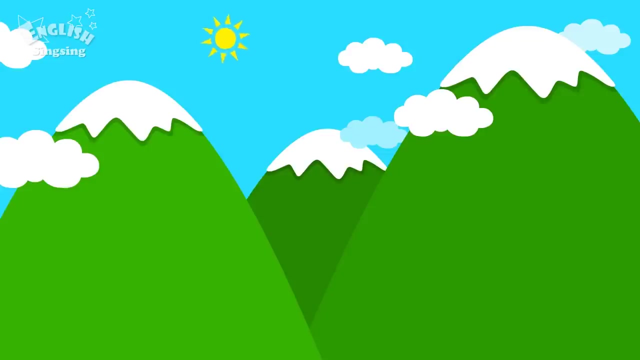 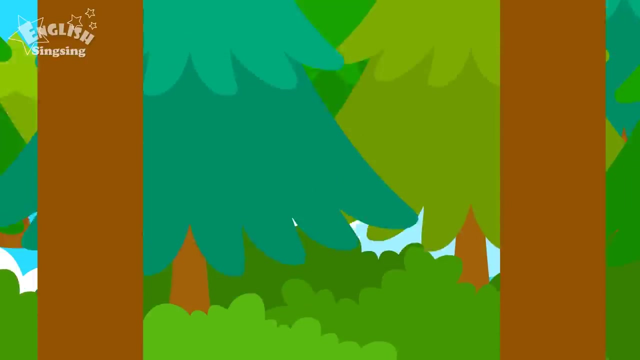 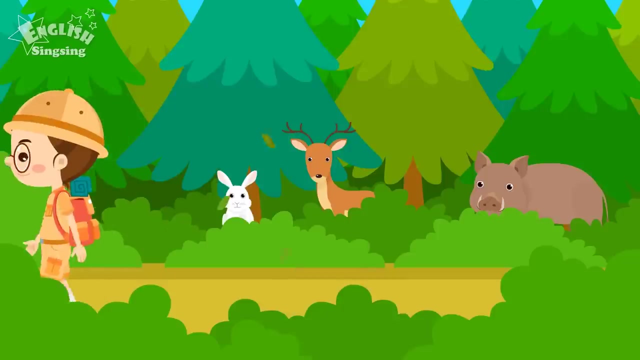 English Singsing: geography: sky- The sky is so high. sky, The sky is so high. land. We are standing on the land, land, mountain, The mountain shoots up, The mountain shoots up. mountain, mountain, mountain, forest, forest. Many animals live in a forest. 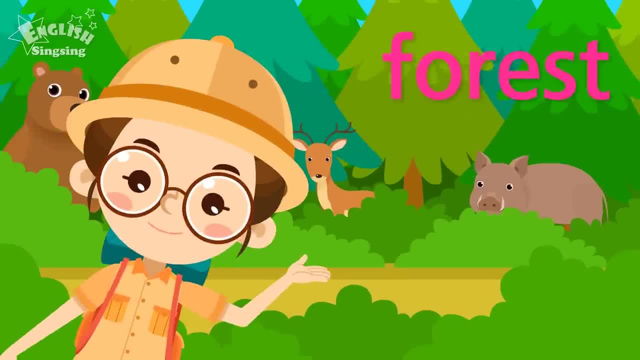 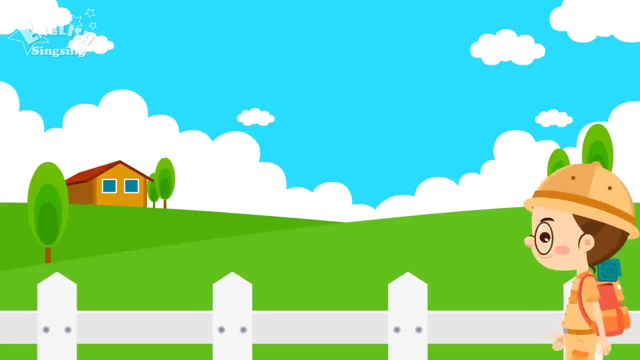 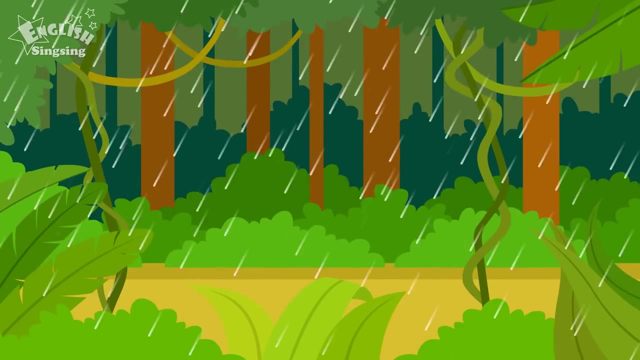 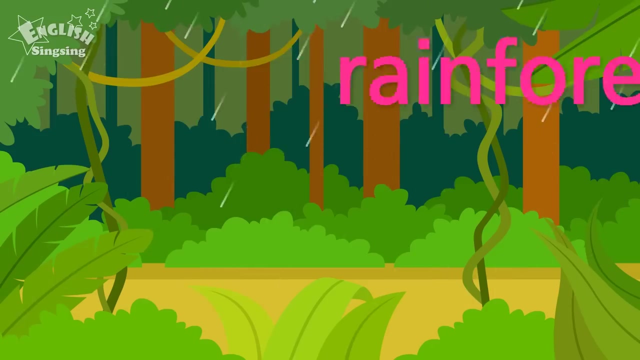 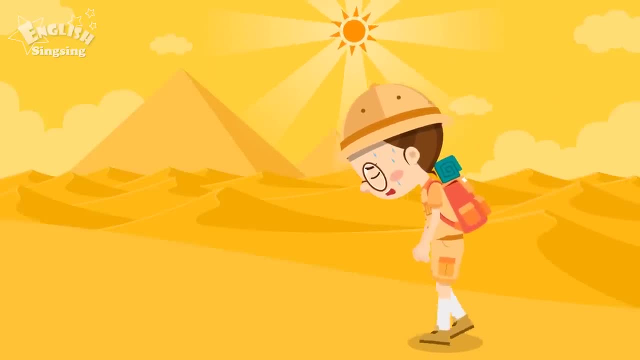 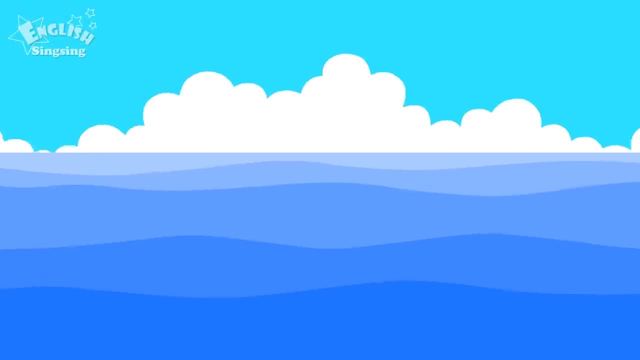 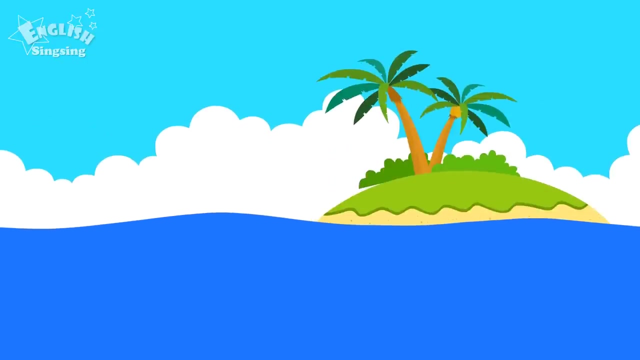 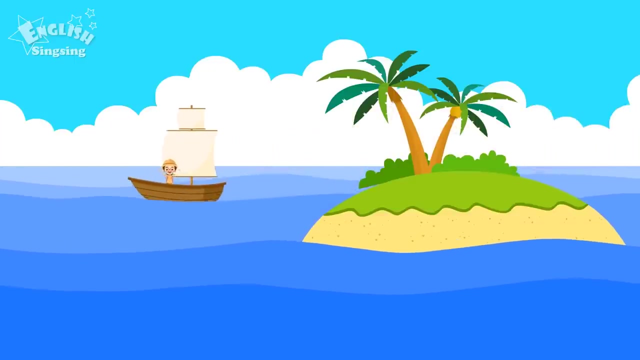 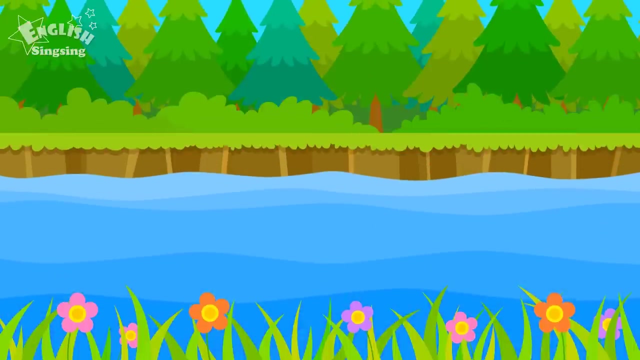 desert. A desert is a very hot and dry place. desert is a very hot and dry place. desert sea: The sea is very deep and blue sea island, An island, is surrounded by the sea island. river river: A river flows into the sea river.